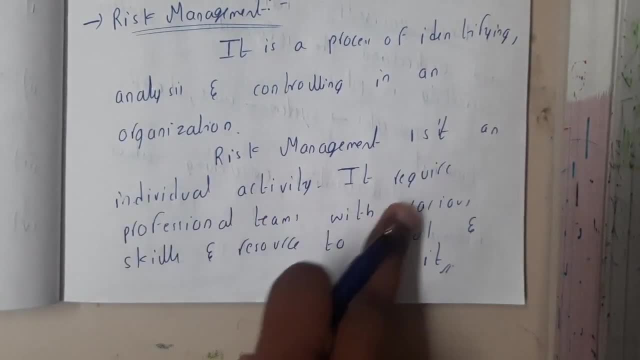 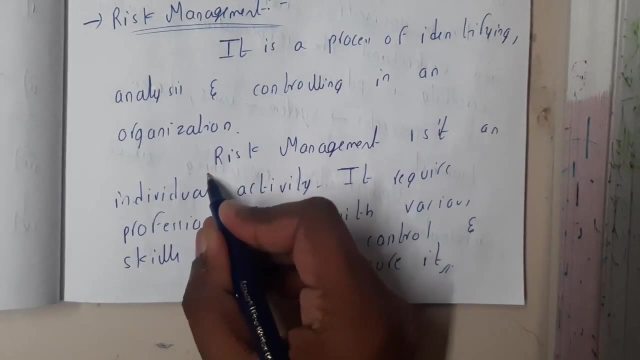 management. Risk management isn't an individual activity. It requires a professional team with various skills and resources to control and secure it. Okay, so, whenever you hear the risk management, okay. So there will be one officer who will be observing everything and there will be one more officer who will be executing everything, and 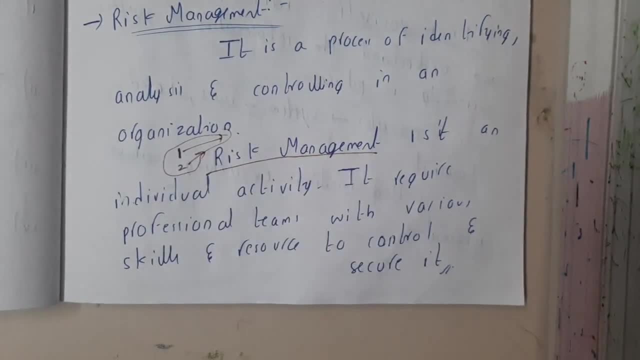 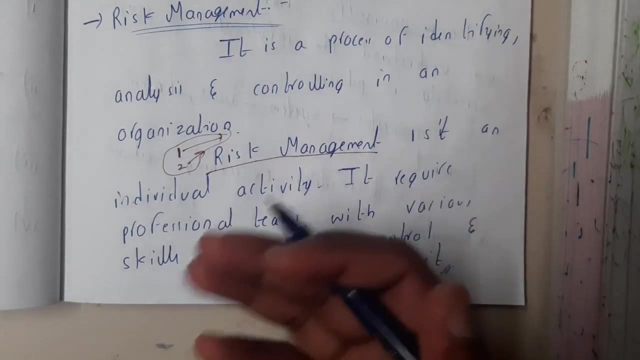 the risk management is done. You have to think in this way. But in large companies, in a high scale companies, there will be having a particular team guys with the many members They'll be doing the analysis and all those things will be done by a team, right, So that? 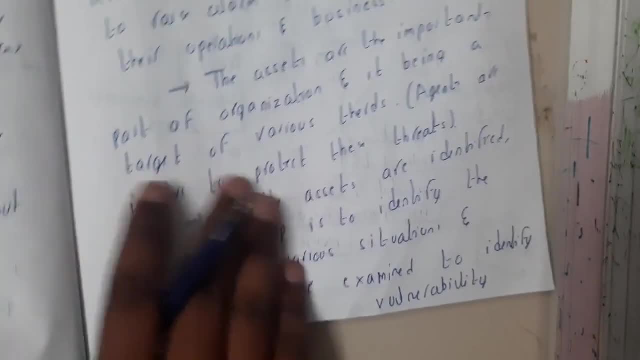 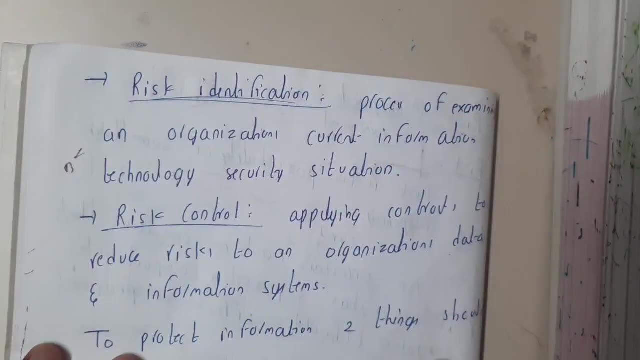 is the scale of risk management as that much important? It is because if it there is a no proper risk management, Then if there is any kind of risk, there will be a huge loss for you. there will be no, no resolving solution, right, yes, okay, so the 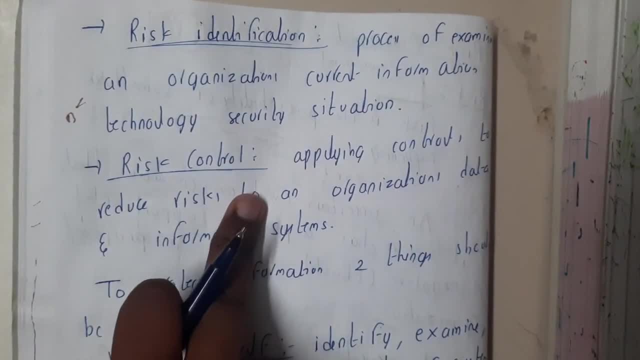 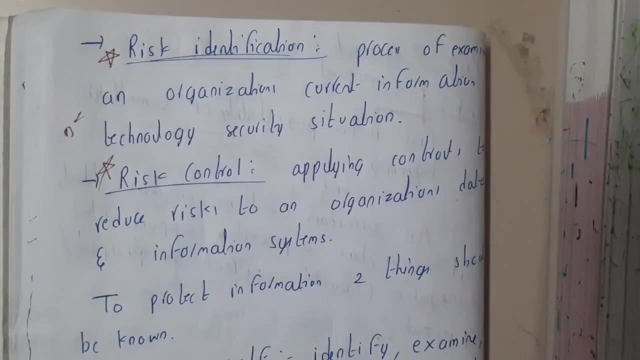 first step is nothing but a risk identification. after that, you'll be doing risk control, okay, okay. please remember one thing, guys: there will be a dedicated video for risk identification and risk control, like next to next. both lectures will be after these two guys. okay, yes, so process of. 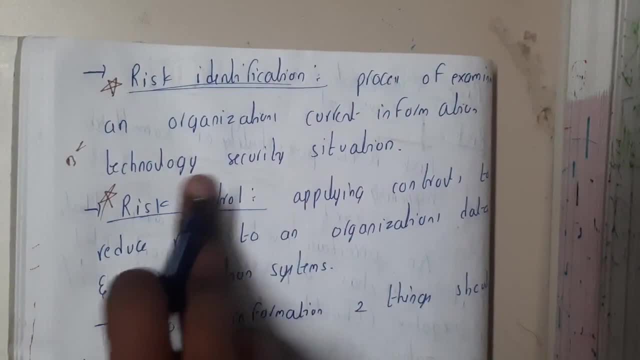 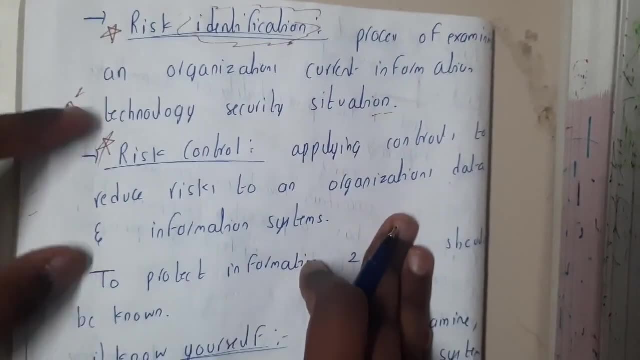 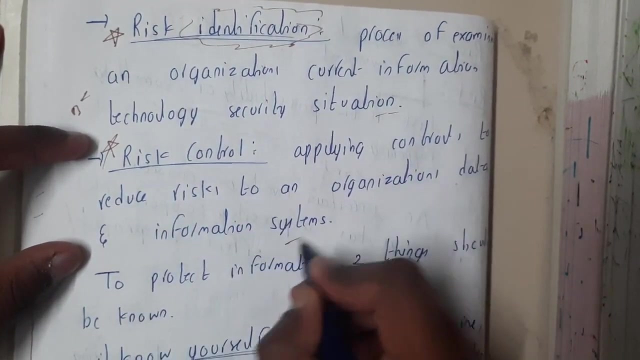 examining an organization: okay, current information technology and security situation. so you will be analyzing everything. so here, by the name identification only, you should understand it, okay. similarly, risk control: so you're controlling it. so applying control controls to reduce the risk to an organization. data. that is nothing but your risk control, okay. so basically, before going into, 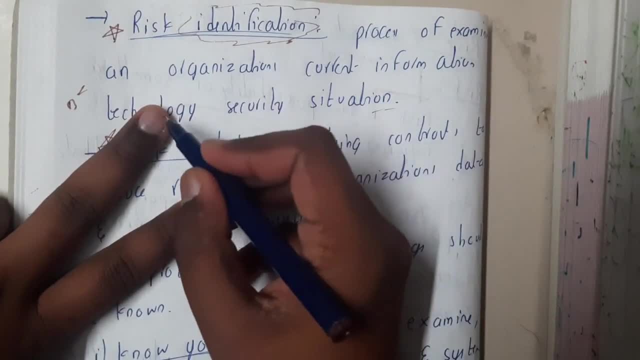 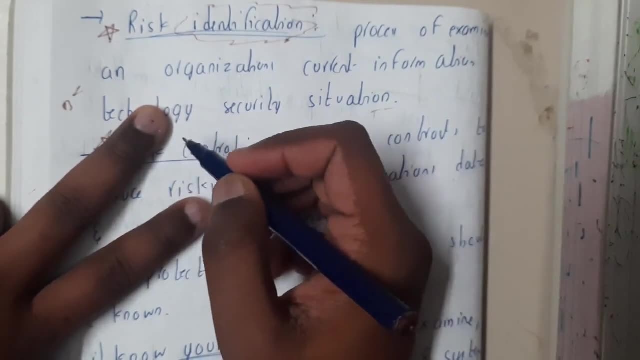 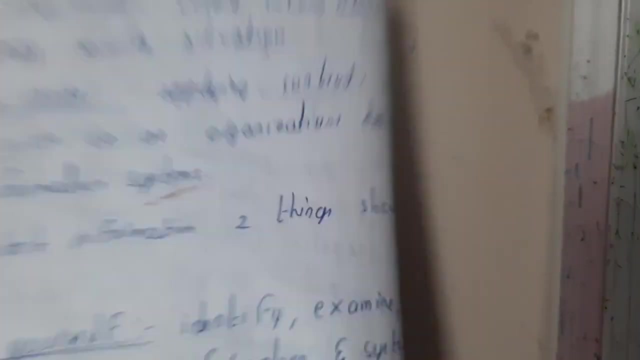 risk. you should know two things, guys. so you should know about yourself who you are first of all. are you a company, are you an organization, are you a member, are you the ceo of the company, or who are you and who can attack you? that is nothing, but who the attacker is, know about the enemy, yes, okay. so if you take some kind of 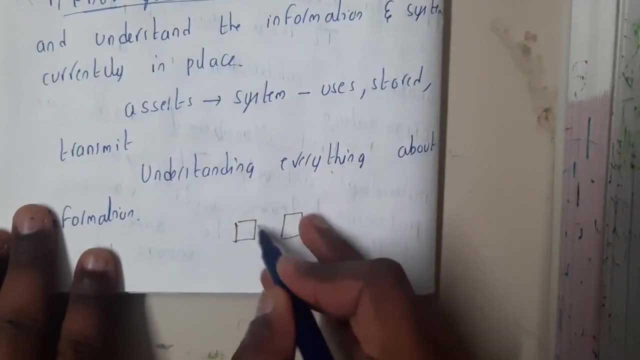 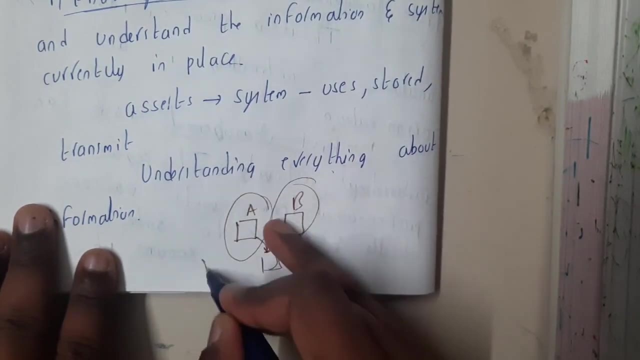 examples, like in companies: so one company and the other company, so this company and this company b, and they are competing for some project, assume in that way right. so before giving their bits they will be knowing that how much the opponent could give, how much they are willing to do like that.